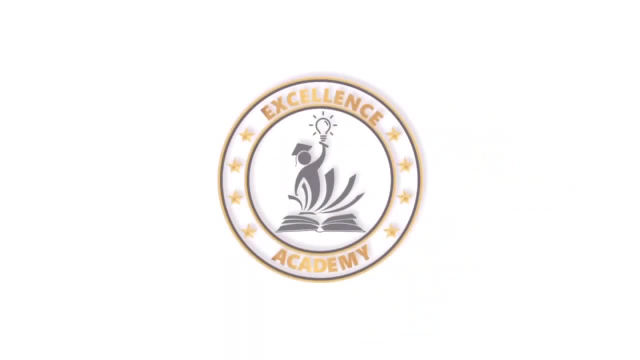 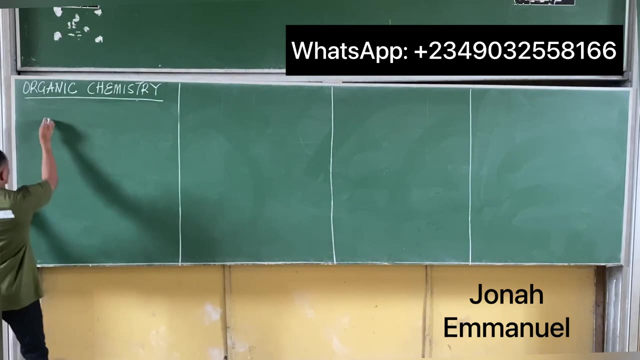 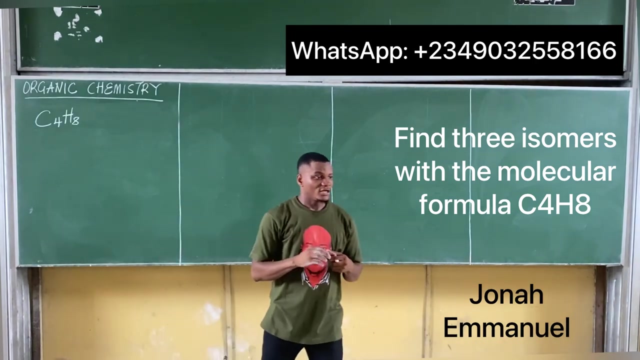 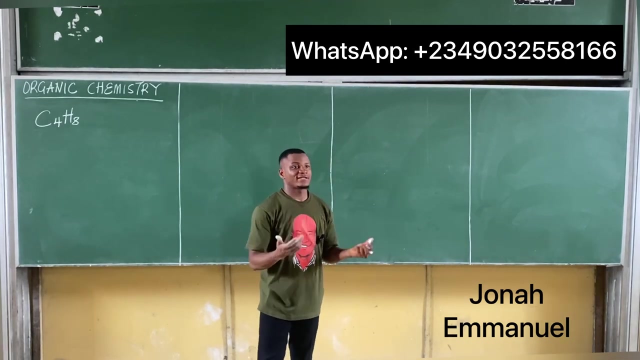 The question on there says you should find what there, The isomers of what there C-what Find the isomers of C4H8.. This person find how many isomers? Find three, All right, so listen, listen, Here's another thing you most likely see in the exam: the concept of isomerism. We said 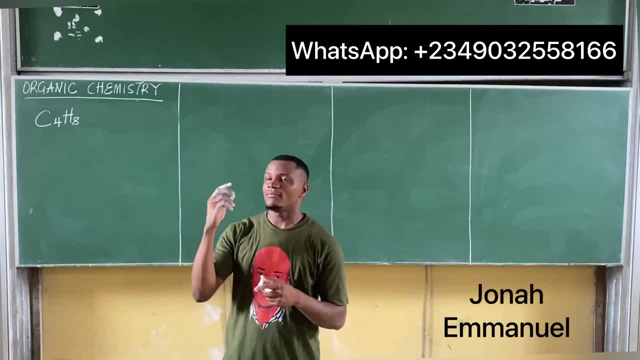 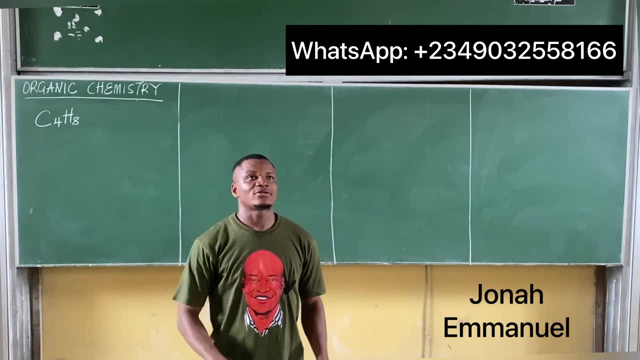 for isomerism. that it's of course, when I have a particular molecular formula, having what there Different structure. That's the idea. So what I'm saying is this: Provide three different compounds, perhaps with three different structure that has the same molecular formula. So how do I do that? 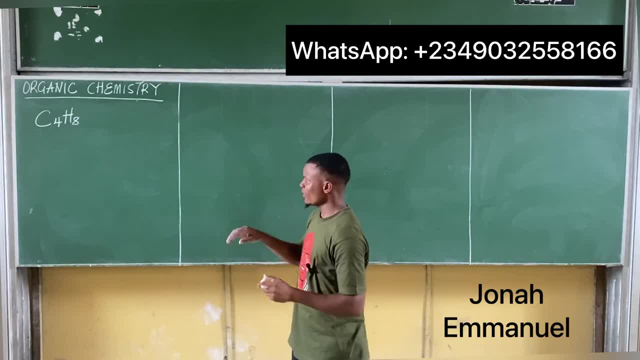 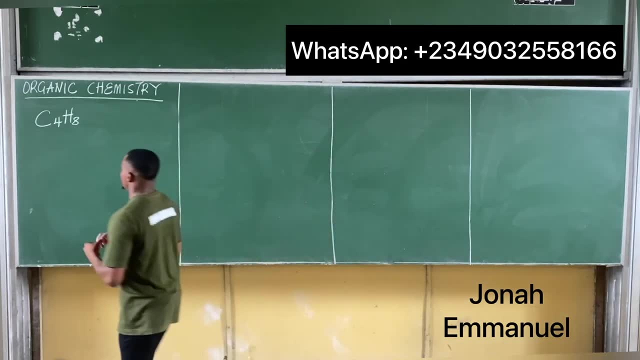 First things first identify what's involved here. When you have C4H8, this time you have the isomers and alkene, alkene or alkyne- Obviously alkene, because I know for alkene my molecular formula is C4H8.. So what I'm saying is that I have a particular molecular formula. So what I'm saying 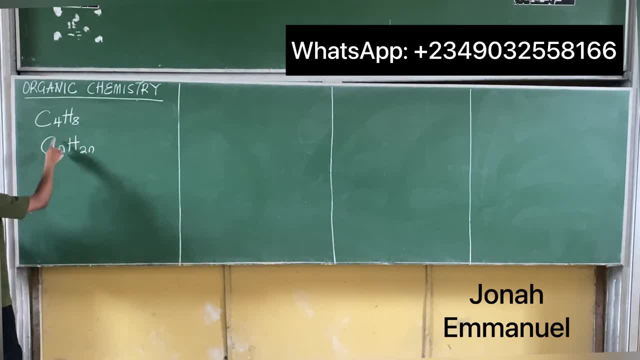 is C4H8.. So hence, if N is 4, that becomes 2 times 4, that's 8.. That means this stuff here is quite alright as an alkene. So my first task will now be create an alkene of what there- 4-carbon That's. 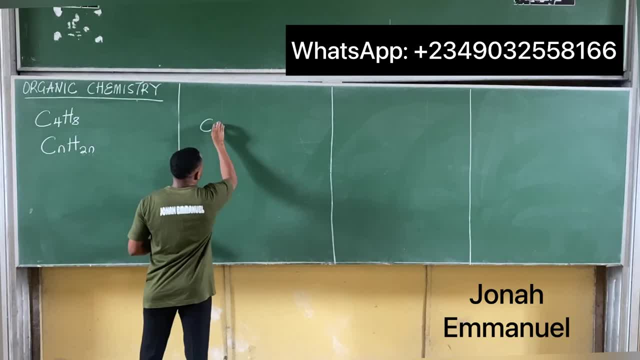 your first task. So it becomes 1,, 2,, 3, 4.. It's at your own discretion to put the double bond anywhere. Don't forget: if I put double bond here, it becomes 1,, 2,, 3,, 4.. If I put double bond here, it becomes 1,, 2,, 3,, 5.. So that's the first task, Then after that, 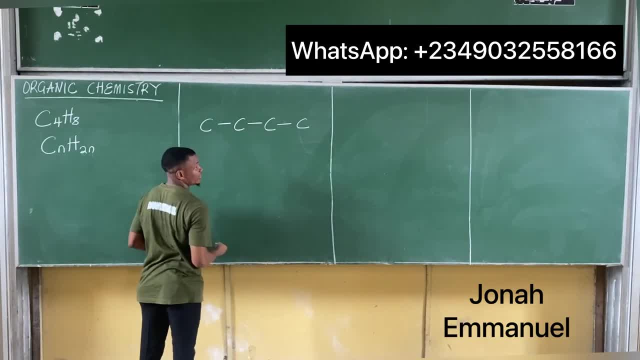 in. If I put double bond here, it becomes 2 in. Whether I'm using 1 in 0 or 2 in 0 is left for you. For me, I am choosing to use 1 in. That means I'm choosing to place my 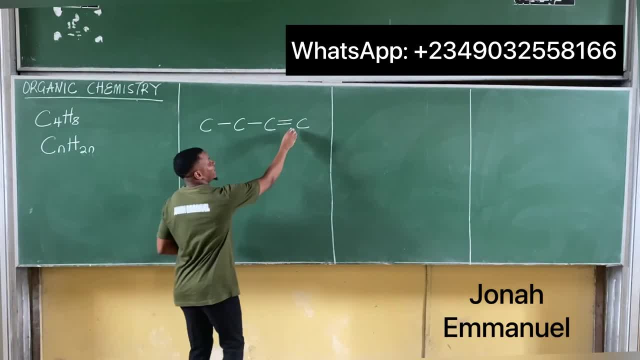 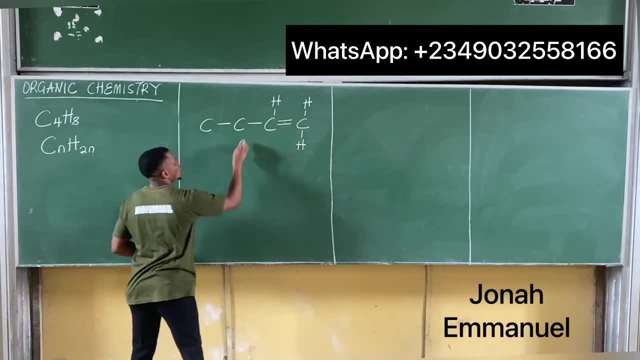 double bond here, So try to complete the structure. This one has 1, 2.. I have 3 and 4.. This one has 1,, 2, 3.. I have 4.. 1,, 2,, 3 and 4.. 1,, 2, 3 and then 4.. I have this, The attack here. 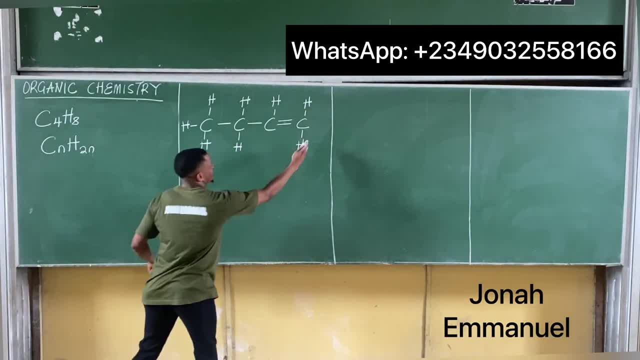 is simple. Try to name this compound. Obviously, I'm going to be numbering this way because I want the smallest number attached to my double bond. So I'm having 1,, 2,, 3, 4.. 4 carbon compound- is what? there A boot, So it becomes boot, Boot 1 there, Boot 1. Boot 1. Boot 1.. 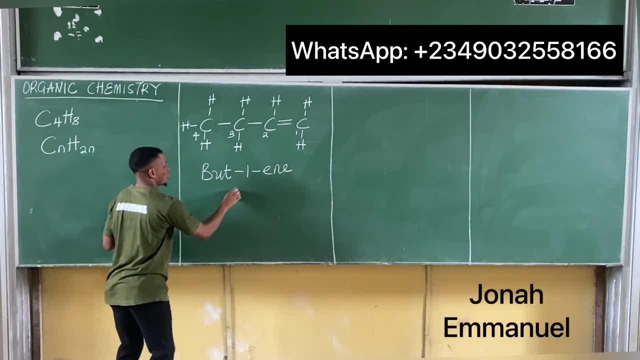 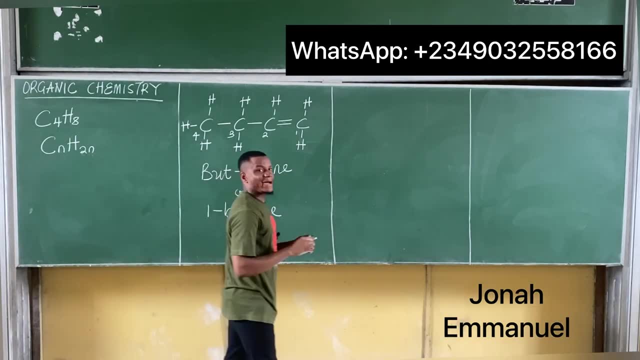 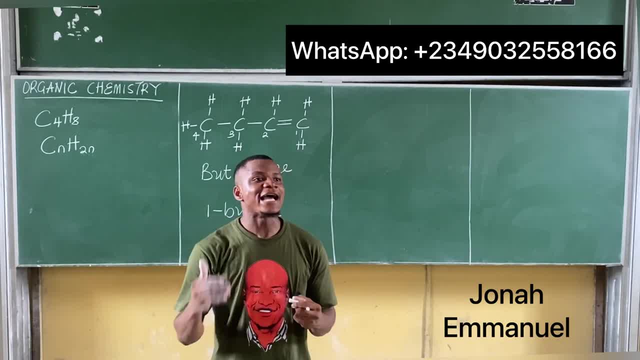 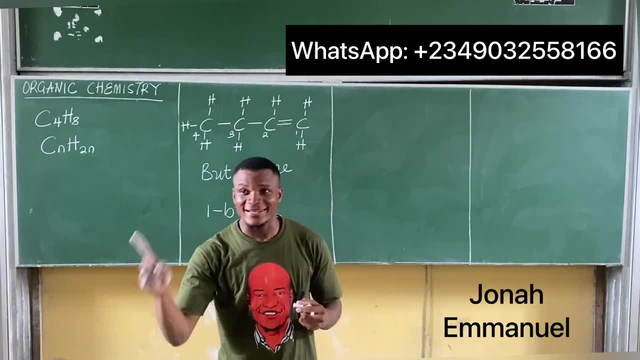 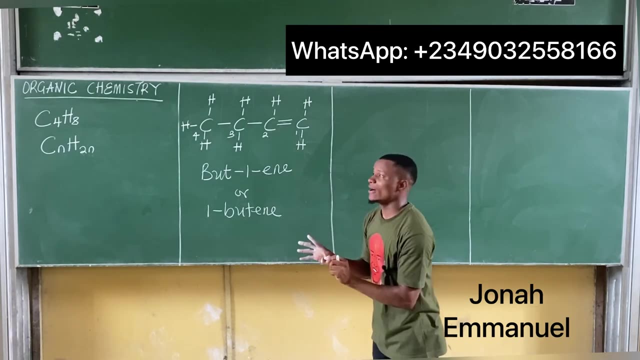 In our last class we said: alkenes are isomers of what? Do you remember? They are isomers of what? there? Cycloalkene. I stressed it. That means for every alkene, each isomer has to be a cycloalkene. So I'm going to form a cyclo compound, Since I'm having four. 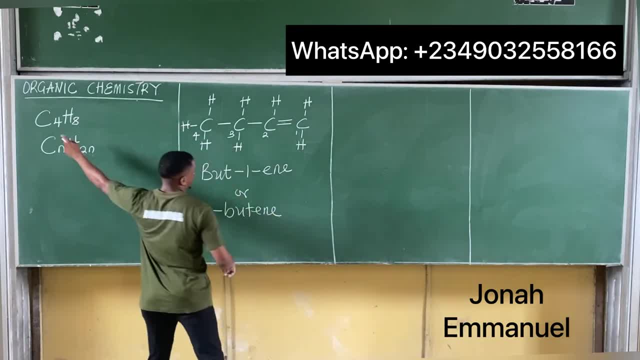 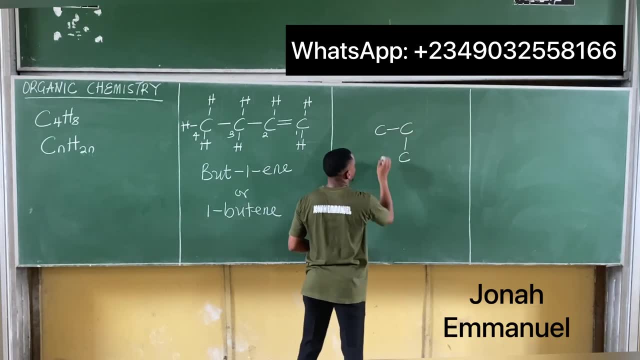 carbon compounds, four carbon atoms per se, I'll form a cyclo compound that has four carbon atoms, So that has to be 1,, 2,, 3, 4.. I have this. Try to balance this out. I'm. 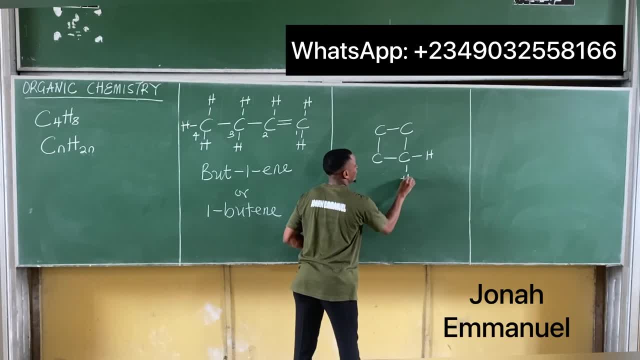 having this as 1,, 2,, 3, and 4.. 1,, 2,, 3, and 4.. 1,, 2,, 3, and 4.. Finally, 1,, 2,, 3, and 4.. 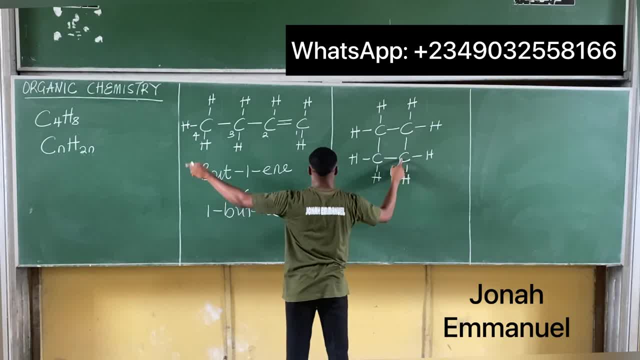 If I count this, 1, 2,, 3, 4,, that's C4.. 1, 2,, 3, 4, 5, 6,, 7, 8. C4H8.. That matches. 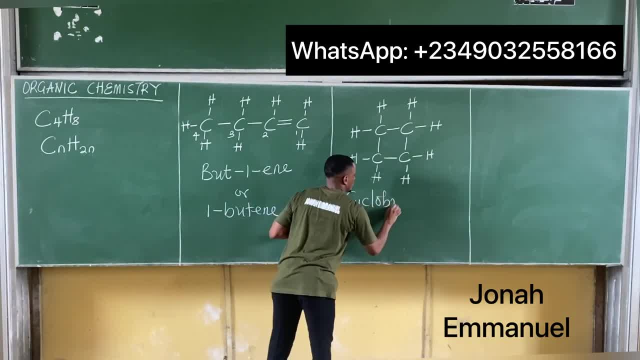 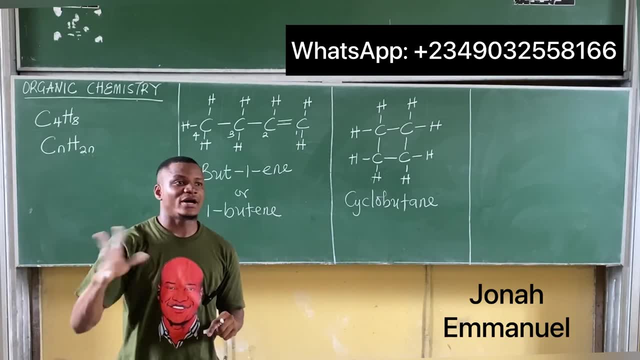 So if I name this compound because what there? Cyclobutane- We are asked to name three. We've worked with the two. we know an alkene and it's isomeric cycloalkene. So what's the third? 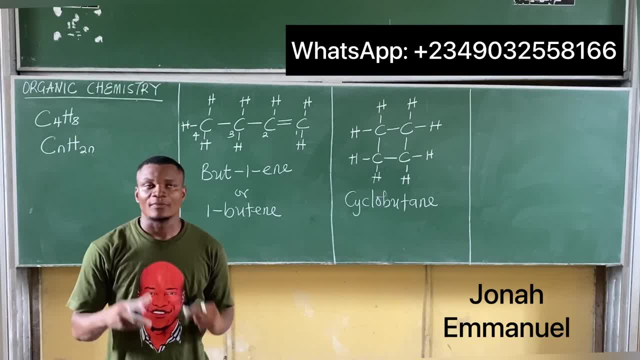 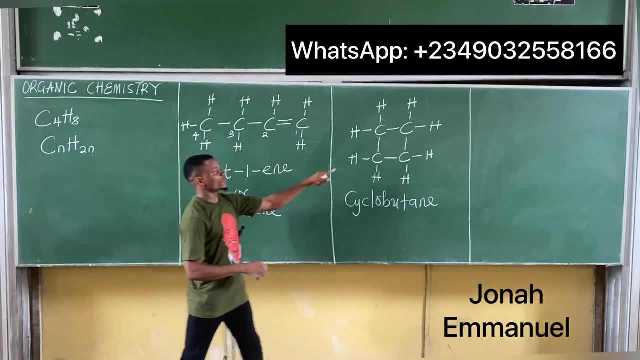 one there. The third concept would be this: As much as you can see, listen please. here's the logic. As much as I can, I used four carbons here. I used four here. We know about these two. Your next task would be: what if I use a three? 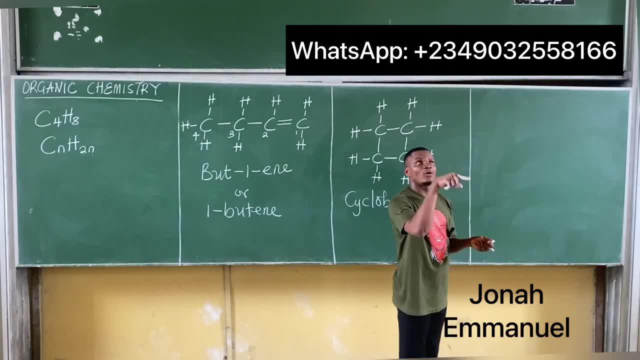 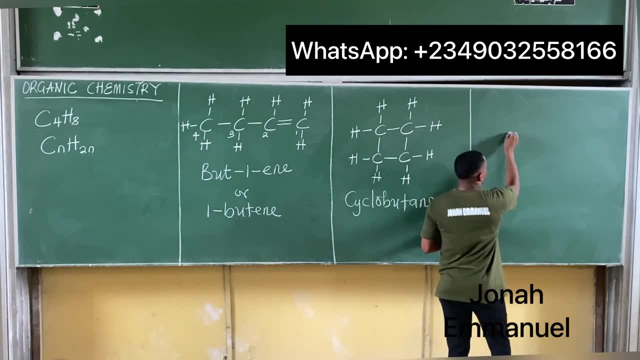 carbon compound and take the fourth carbon compound as a substituent. That's the idea. So instead of using four, now use three, So 1,, 2, 3.. I have this, Place the fourth carbon compound as a substituent and see if it balances out. Now I'll place the next one here here. to make it four, Of course, my longest continuous carbon chain has to be 1,, 2,, 3,, 4,, 5,, 6,, 7,, 8,, 9, 10,, 11,, 11,, 13,, 12, 13.. 1,, 2,, 3,, 4.. 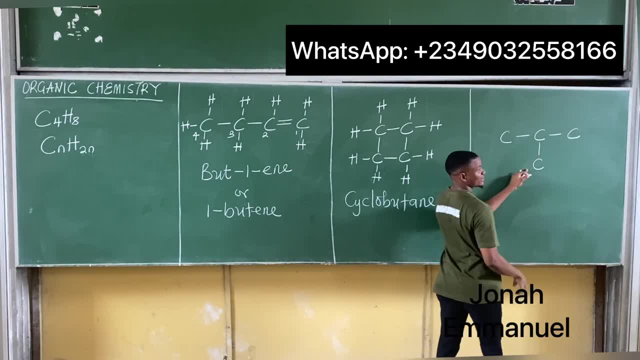 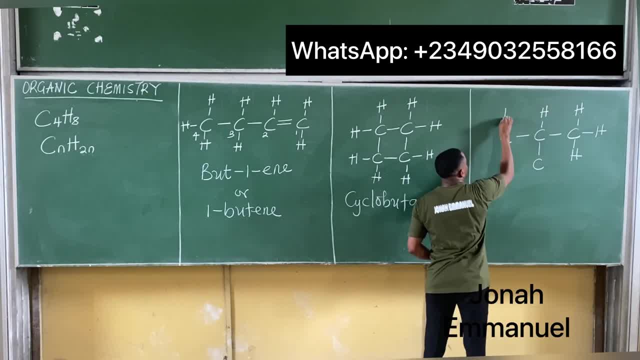 1,, 2,, 3,, 4.. So if I count, I have 1, 2,, 3,, 4.. So carbon 1, 2, 3,, 4,, 5,, 6,, 7,, 8.. 1, 2,. 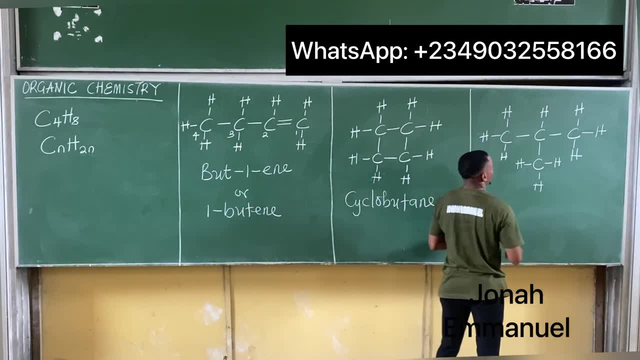 3, 4.. So if I count, I have 0.5, 3, 4, 5.. Okay, so thisÜ is a. It's called U Yes, six um one, two, three, four, five, six, seven, eight, nine. okay, it doesn't work, but that's not it. 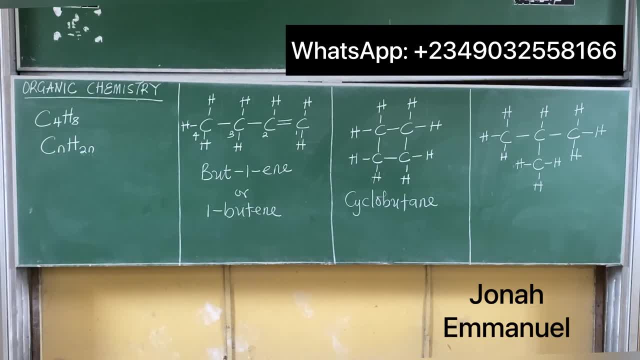 uh, let's try to see if i use a double bond instead. so what if i look at this? this is the work now. what if i try to use a double bond instead? that means, let me form a double bond that this. so look at this now it becomes: uh, one, two, three. 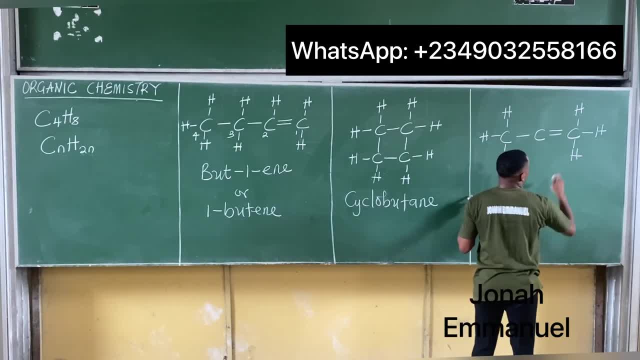 let me add double bond here. so i have this. so this now becomes one, two, three. this one is balanced: one, two, three, four. this is uh, nope, it's wrong. so take off this one here. so it becomes one, two, three, four. uh, that's quite complete. i'm having one, two, three. one, two, three, one is left. so here c: one, two, three. 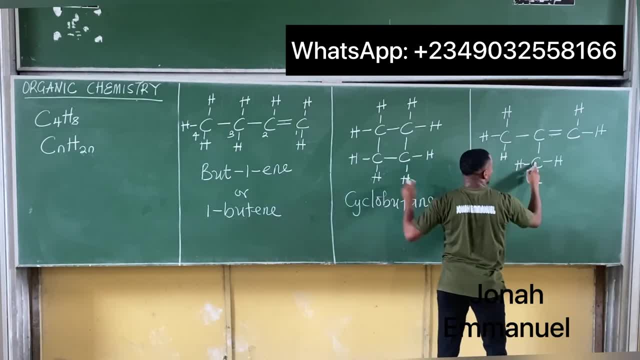 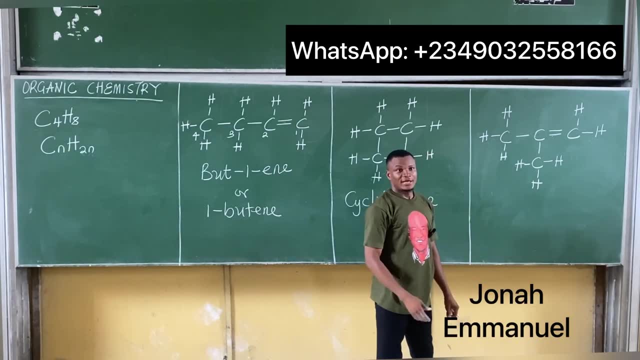 all right. so if i now count, i have one, two, three, four, c four. one, two, three, four, five, six, seven, eight. that's correct. so see the way i worked with this. i tried to see single bond. it was more than required and i used double bond and the subsequent. it worked. so how do you know this?